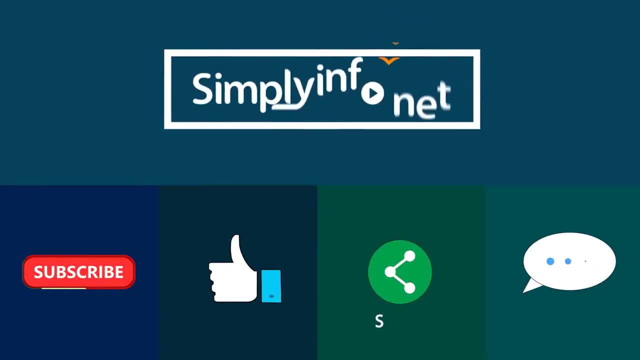 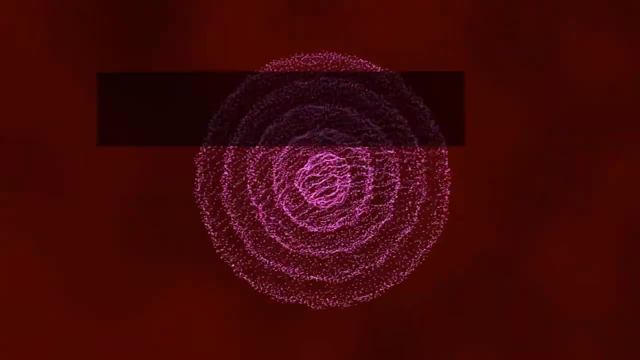 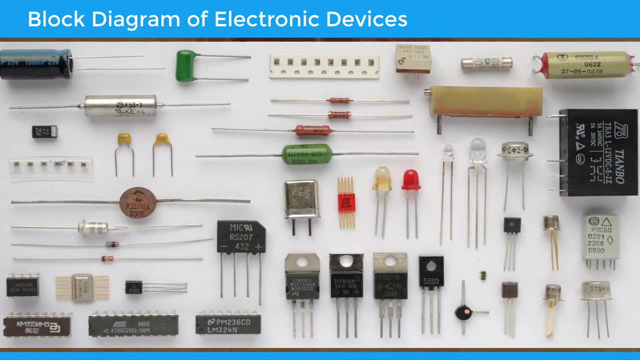 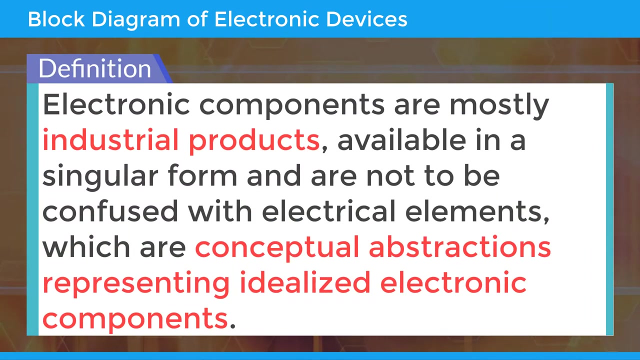 Block diagram of electronic devices. Electronic component definition. An electronic component is any base, discrete device or physical entity in an electronic system used to affect electrons or their associated fields. Electronic components are mostly industrial products available in a singular form and are not to be confused with electrical elements which are conceptual. 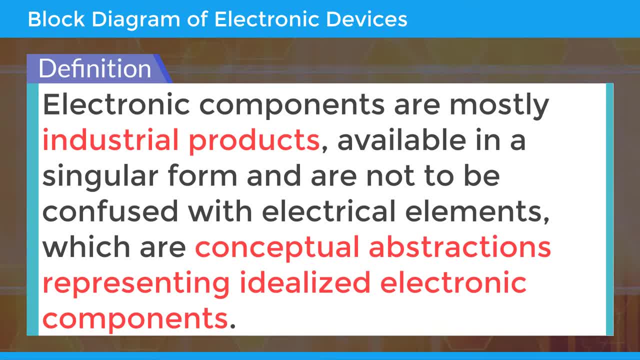 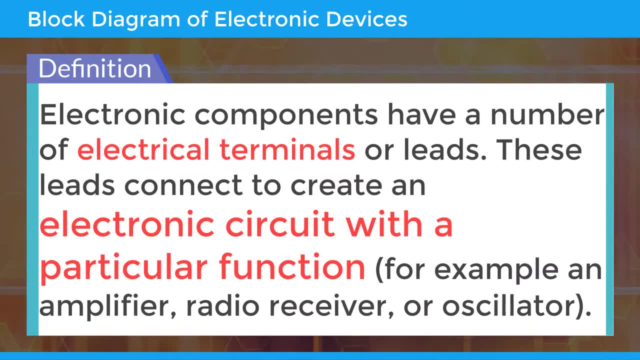 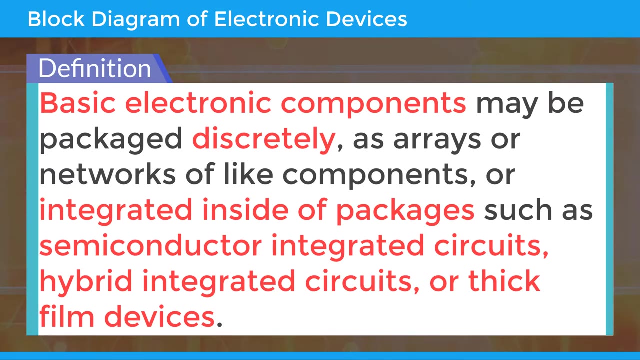 abstractions representing idealized electronic components. Electronic components have a number of electrical terminals or leads. These leads connect to create an electronic circuit with a particular function, For example an amplifier, radio receiver or oscillator. Basic electronic components may be packaged discreetly as arrays or networks of like components, or integrated inside. 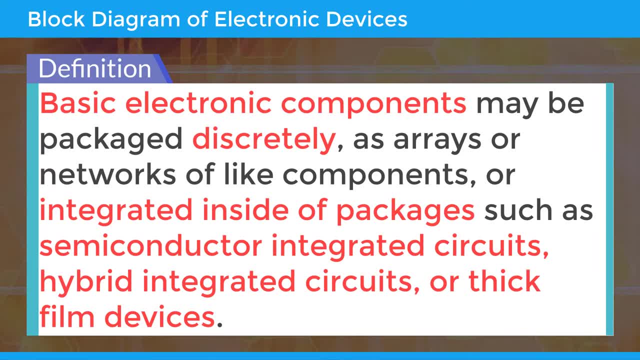 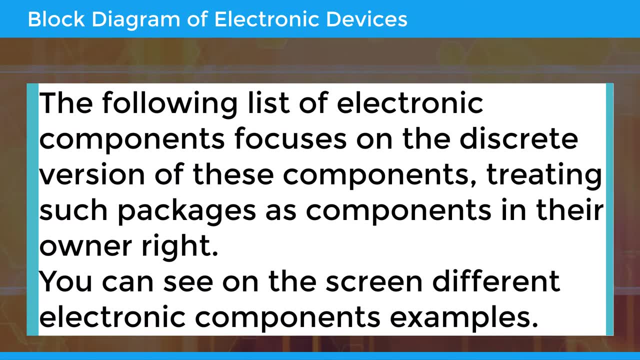 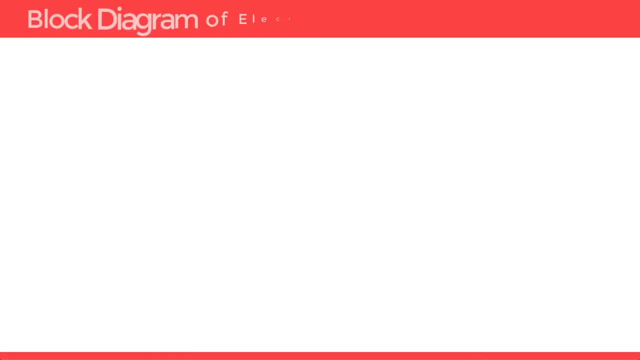 of packages such as semiconductor integrated circuits, hybrid integrated circuits or thick film devices. The following list of electronic components focuses on the discrete version of these components, treating such packages as components in their own right. You can see on the screen different electronic components. examples: Block diagram: Electronic components are divided into: 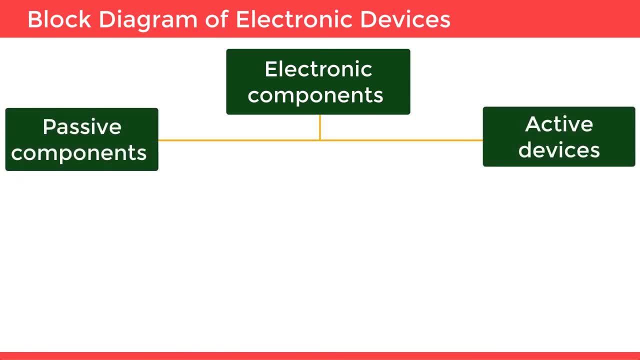 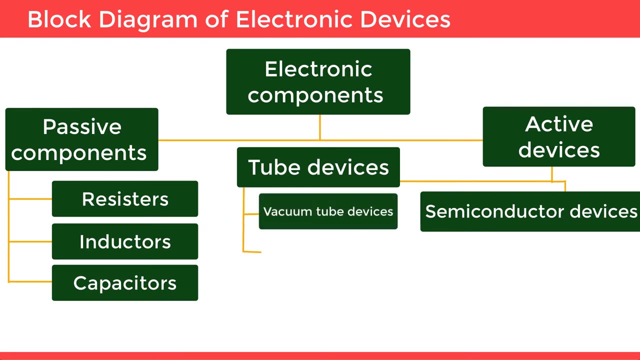 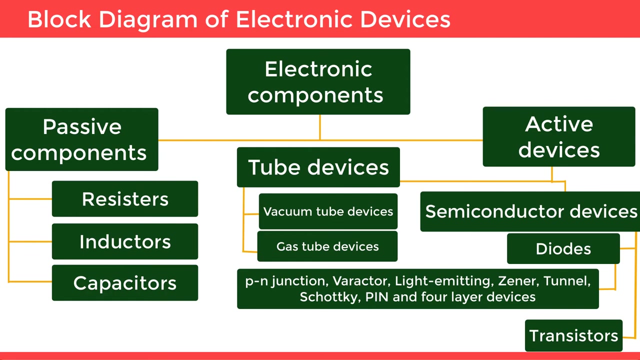 two types: Passive components and active devices. Passive components includes resistors, inductors and capacitors. Active devices are divided into tube devices and semiconductor devices. Tube devices includes vacuum tube and gas tube devices. Semiconductor devices includes diodes and transistors. Diodes includes pn junction, varactor, light emitting zener tunnel, shorty pin and. 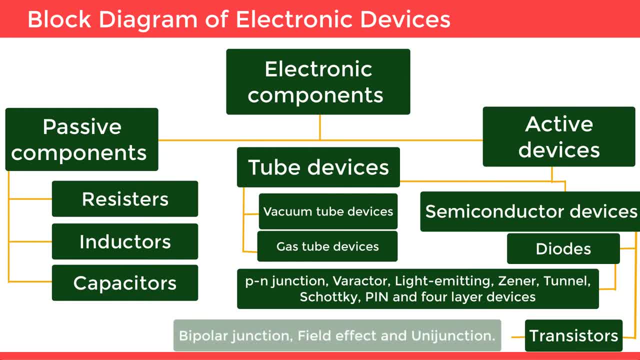 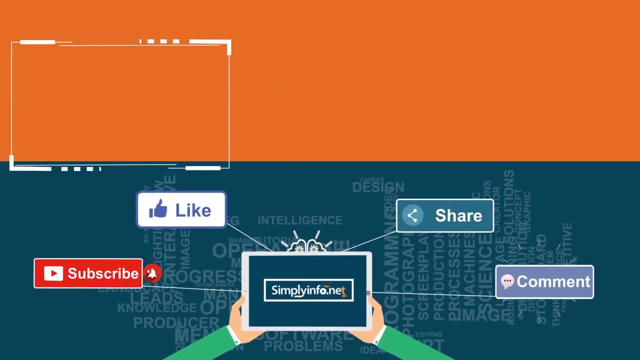 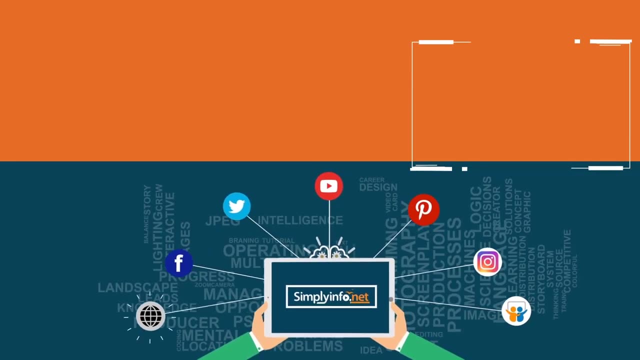 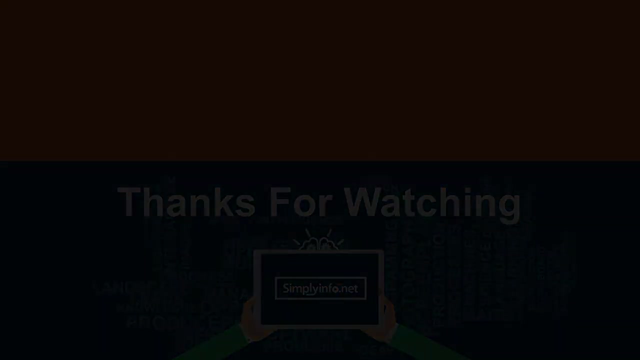 four layer devices. Transistors includes bipolar junction, field effect and unijunction. The following list of electronic components is a summary of the components. The following list of electronic components is a summary of the components.